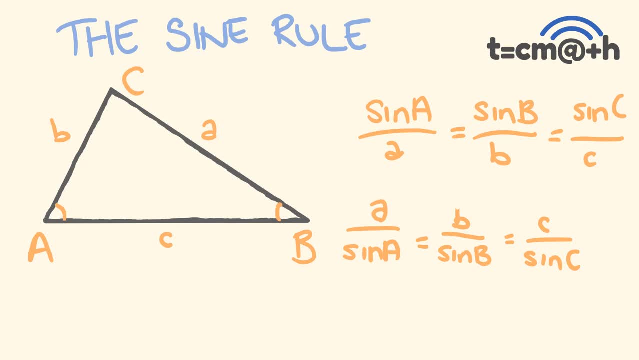 Okay, so I'll show what I mean And I'm just going to reduce this rule here to its most simple by getting rid of all this stuff here. So say, I was just considering sine A and A and sine B and B are angle A, line A, angle B and line B. 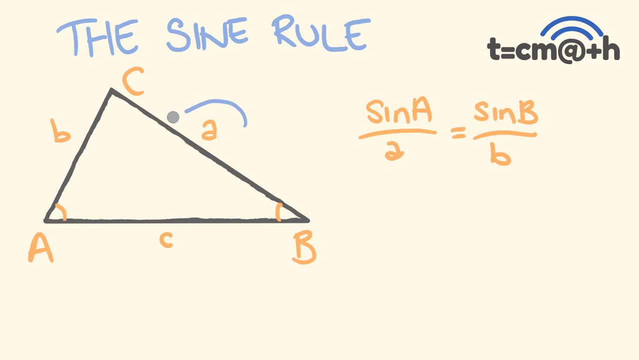 We have two matching sets here. We could use so, say we knew these particular figures here We knew the angle of A and we knew the line length of A here And say we only knew B. We could use this also to work out this particular side length over here. 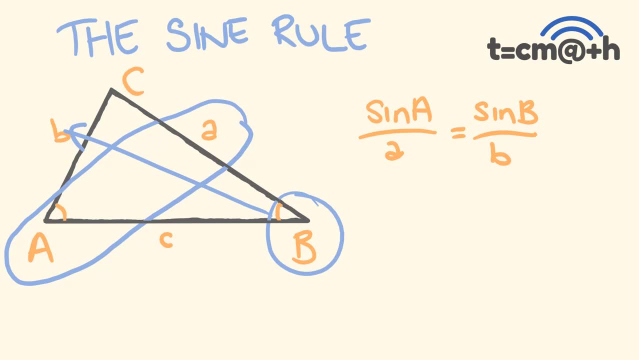 Okay, and that's where the sine rule is really, really handy. As long as we know at least one full set and part of the other set, we can use it to work out the rest Okay. so let's have a look at this in action. 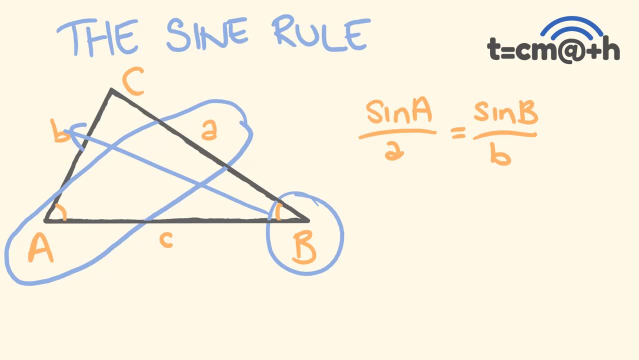 I'm just going to go through two examples. We're going to work out one with the side, We're going to work out one with the angle, And I'm also going to show you just a little trick that you can use within this, just in case you get a particular type of question. 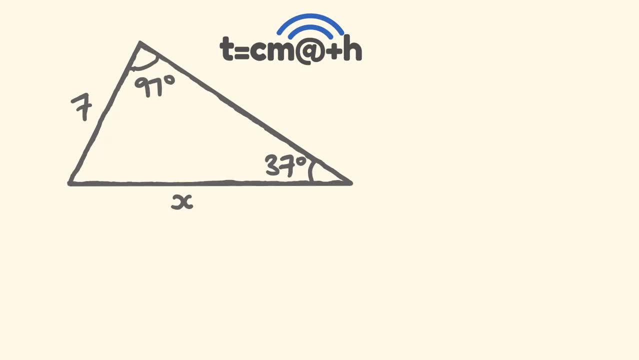 Okay, so Let's have a look at an example here. Okay, for our first example here, we have a triangle where we have an angle of 37 degrees and its corresponding side that opens out to 7.. We also have an angle of 97 degrees, which opens out to a corresponding side that we're trying to find. 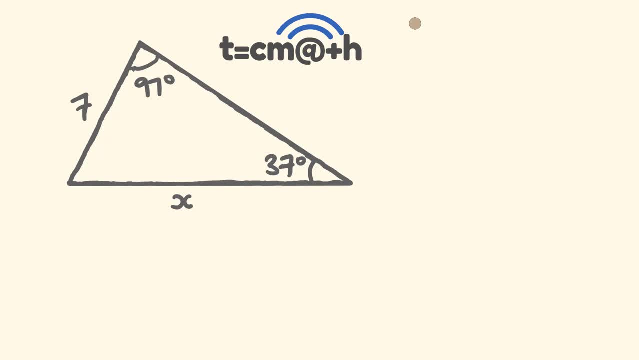 So we're going to use a condensed version of the sine rule as follows. We're going to be using this particular one here: A over the sine of capital A equals B over the sine of capital B. we only need to use this particular part of the song and we don't need to use the whole thing. 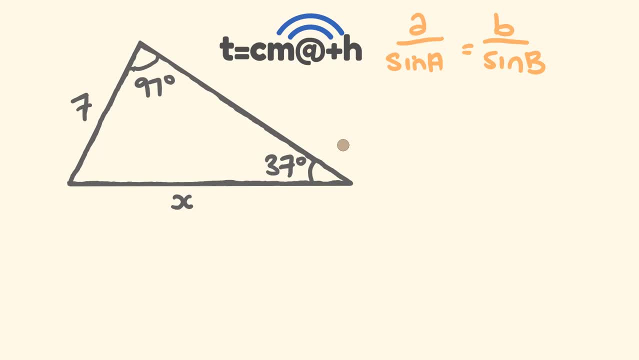 Okay, so let's go through and lay less odds Now. now I'm going to like to keep my unknowns on this side. It's just a little thing I like to do, So let's start with that. We're going to unknowns here, which I'm going to be calling our Asia. 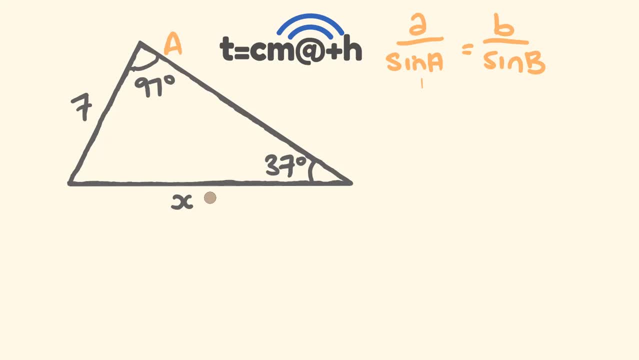 So this is going to be a capital A for our angle and a little eye for our side which goes along with it. We have a capital B for our angle here that we do know, And a little B For that side length here that we do know. 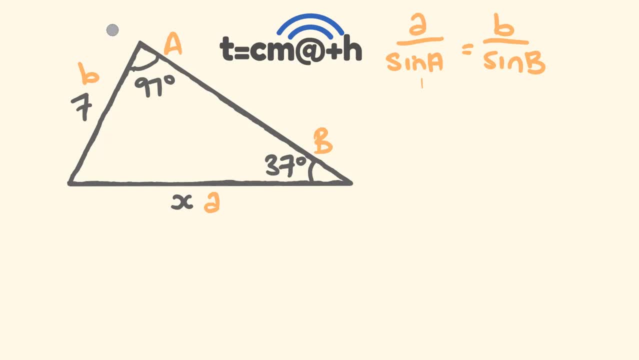 So now let's go through and substitute in our values: Okay, so we have okay, A, which is equal to X. We have sine of 97 degrees. Okay, and this is equal to B, which is 7 over the sine of 37 degrees. 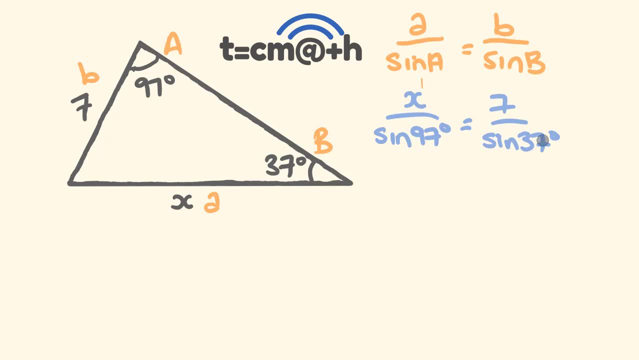 All right Now. we're going to go through now and work out the sine of 97. And the sine of 37. So if we were to do this, we're going to get the following: We're going to get the sine of 97 degrees. 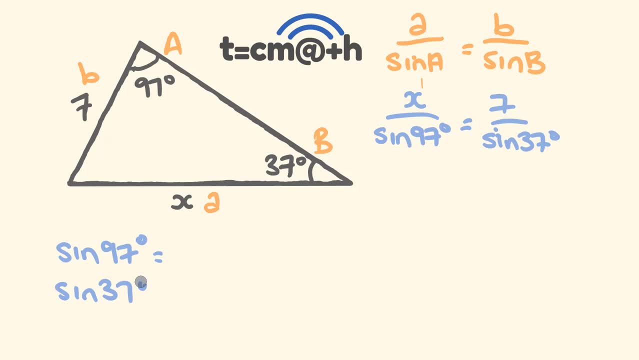 And we're going to work out the sine of 37 degrees, And these are as follows: The sine of 97 degrees is equal to 0.99.. The sine of 37 degrees is equal to 0.60.. So now we can substitute these into our equation here. 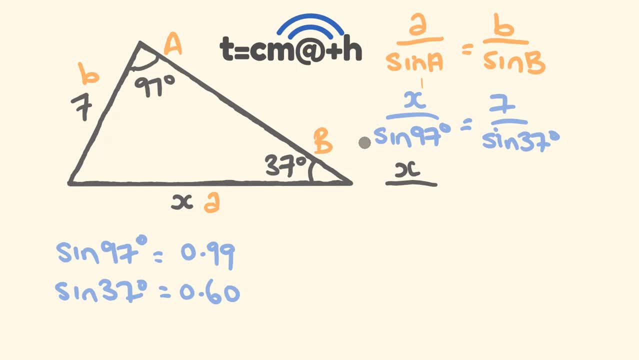 Okay, so we're going to end up with X Over The sine of 97 degrees, which is 0.99.. Which is equal to 7 over the sine of 37 degrees, which is 0.60.. All right, we can solve this particular part here. 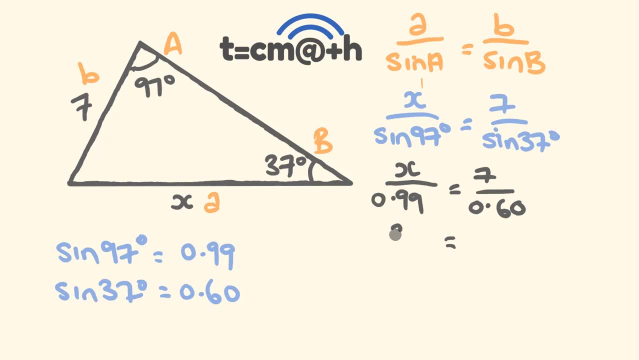 7 divided by 0.60.. So X over 0.99 is going to equal whatever 7 divided by 0.60 is, Which is 11.666666666.. So 11.67.. All right, what do we do now? 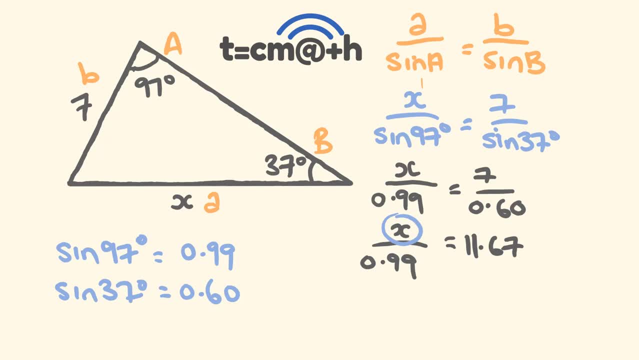 To find X. this is what I usually do. I've done this on other videos. When we don't know what to do, we can go to a friendly equation: 6 over 2 equals 3.. We're trying to find the one at the top here. 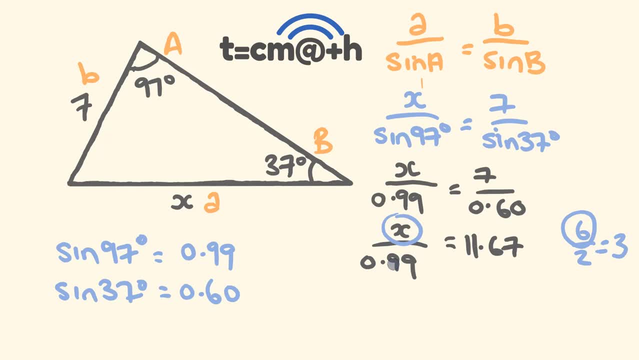 We're going to multiply these, Because 2 times 3 equals 6.. We're going to multiply these two numbers to find out what X equals. So X is equal to this number times this number, Which is equal to 11.55.. 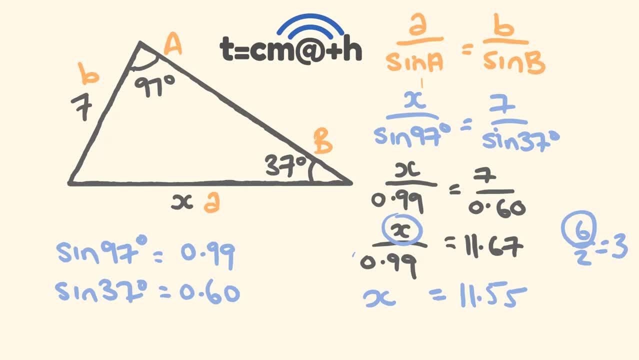 So this particular sine, This particular side here, is equal to 11.55.. And that's how easy it is to use the sine rule. For our next example, we're going to be using a two-step problem Where we're going to find an angle, but there's going to be a little bit of an extra step in there. 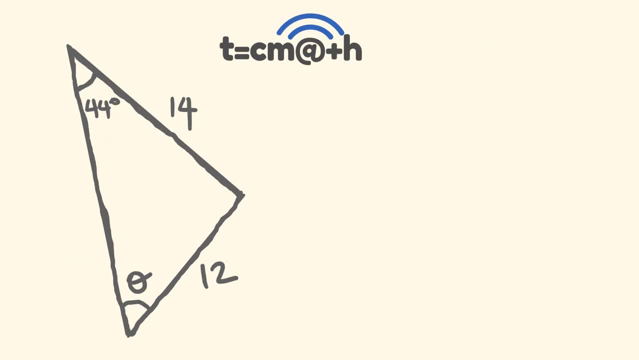 So let's get to that. Okay, for this particular example: here We have a non-right angle triangle. We have an angle of 44 degrees. It opens out to a side length of 12.. We have an angle here that we're going to be trying to find here. 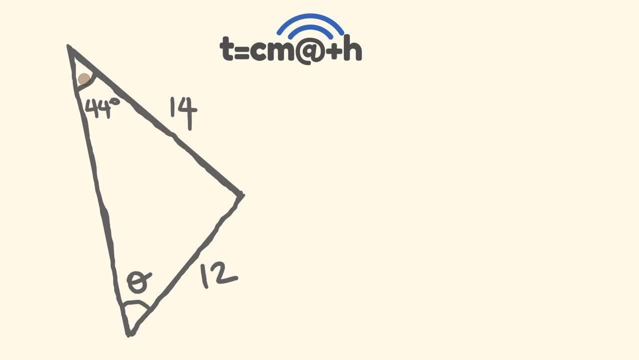 That opens out to a side length of 14.. So we're going to be using the following formula: We're going to be using the sine of capital A over little. a equals the sine of capital B over little b. If it's the angle, I like to use the sine a on top here. 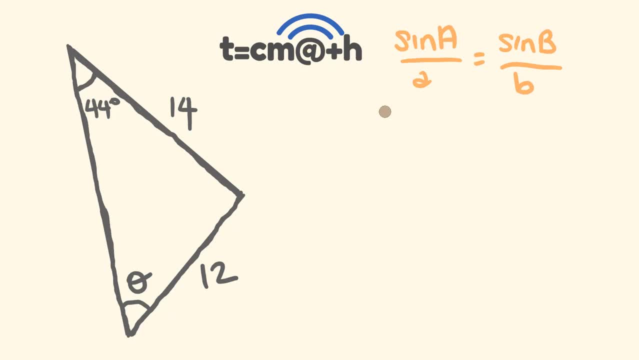 And if it's the side length, I use the little a on top there. So just a little thing Just makes life a whole lot easier, as you'll find out as you go along. So let's work these out. So let's label our sides first, 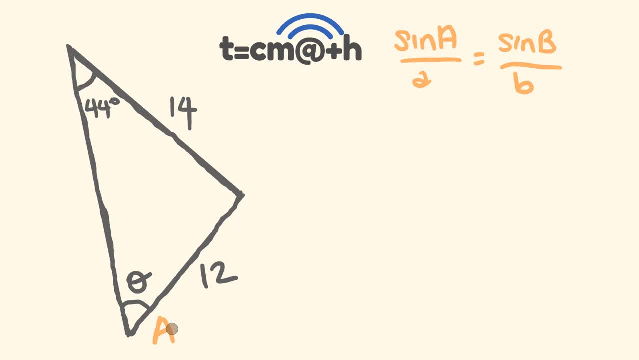 I like to keep the unknowns on this side. So I'm going to be calling this side a and this side little a. I'm going to call this side, therefore, b, Capital b and this side little b. So let's sub in our values here. 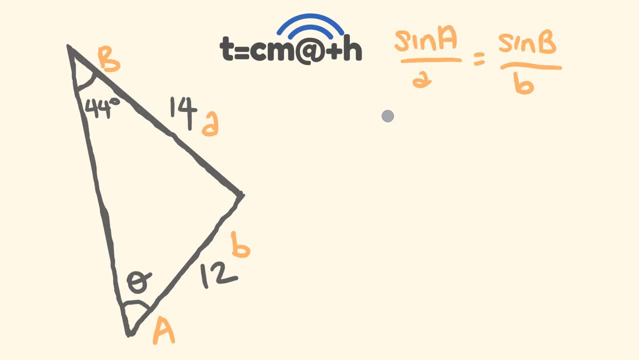 So sine of a is equal to sine theta And little a here is equal to 14.. This is equal to the sine of b, which is 44 degrees, And we're going to put this over little b, which is 12.. So what is first off? the sine of 44 degrees. 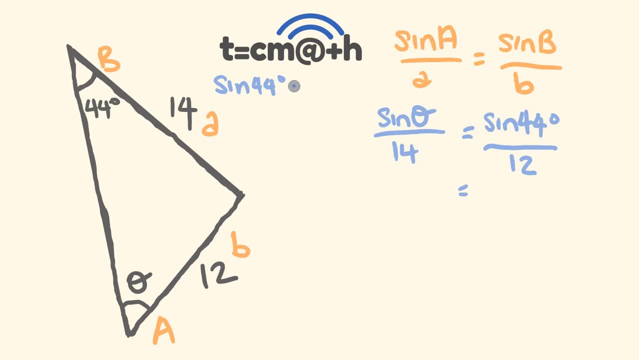 The sine of 44 degrees is equal to- and you can work this out on your calculator- 0.69.. So let's sub this in to our equation. here We have sine theta over 14, which is equal to 0.69 over 12.. 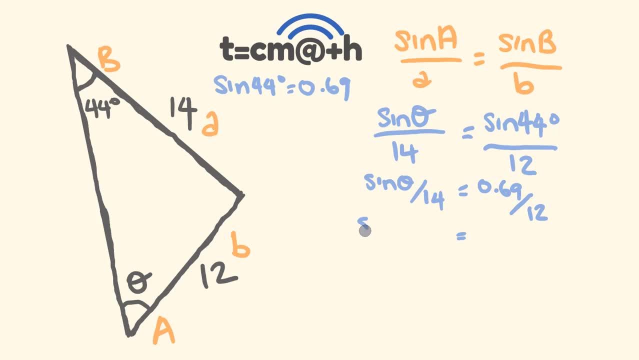 So, writing it all out again now, Sine theta over 14 is equal to 0.69 over 12.. So 0.69 divided by 12 is 0.058.. Okay, so how are we going to solve for sine theta here? 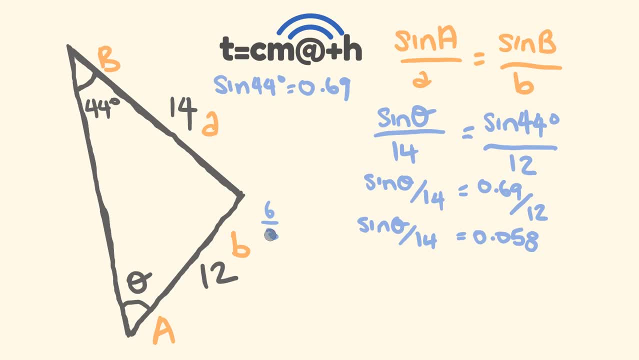 Well, like before, we could do this: old 6 over 3 equals 2.. We're after the number on the top, so we're going to multiply these two numbers. We're going to multiply these two numbers because we're after the number on the top.